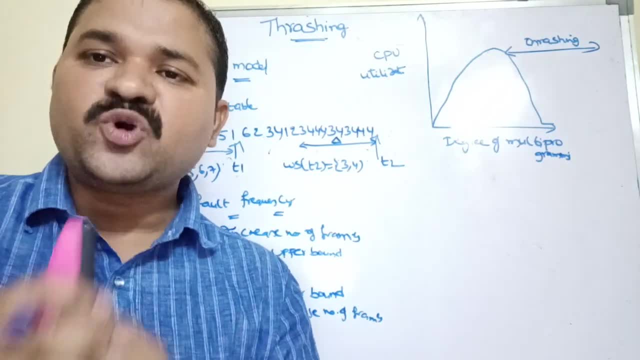 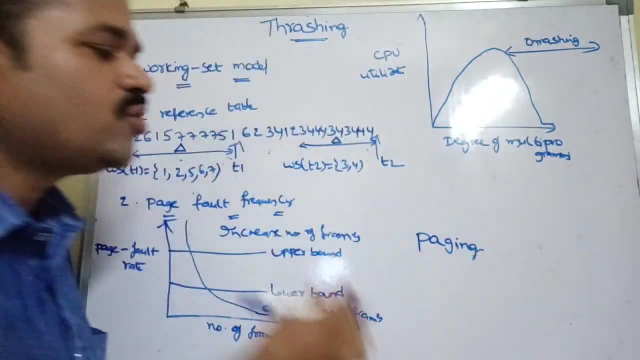 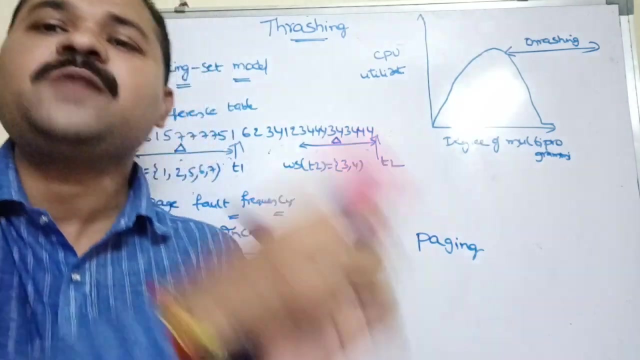 Now let's see about trashing. If a process spends more time on paging rather than executing, then it is known as trashing. Here paging means swapping of pages between secondary memory and main memory. So whenever CPU needs to execute a page, let that page is not present in the main. 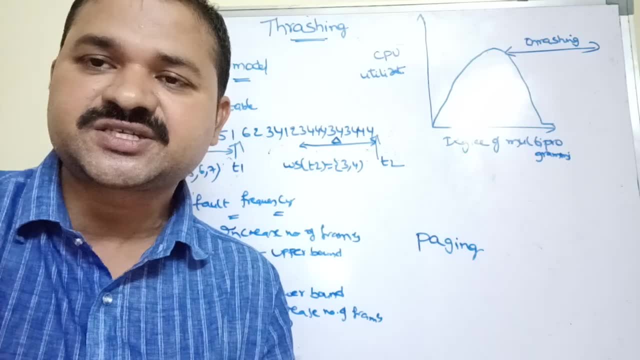 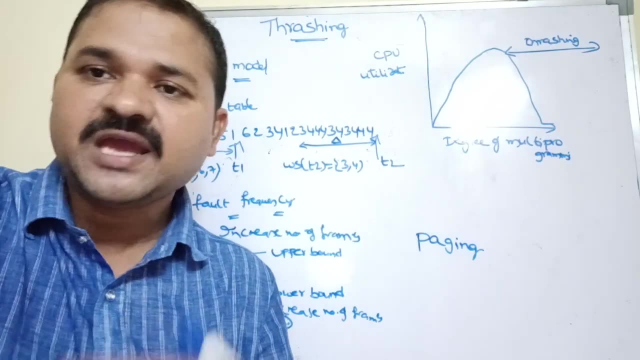 memory. So page fault occurs. So whenever a page fault occurs then operating system has to load that page from secondary memory to the main memory. So, but before that the page in the main memory will be transferred to the secondary memory. So that process is known as paging. So 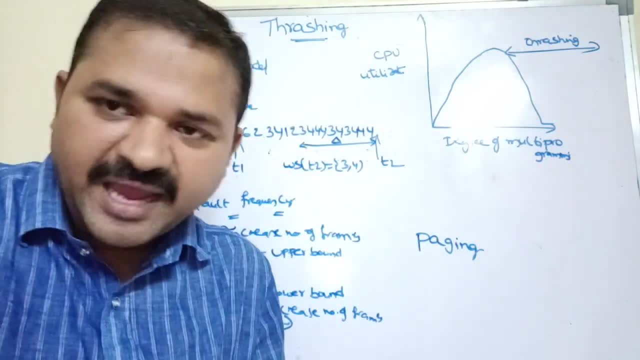 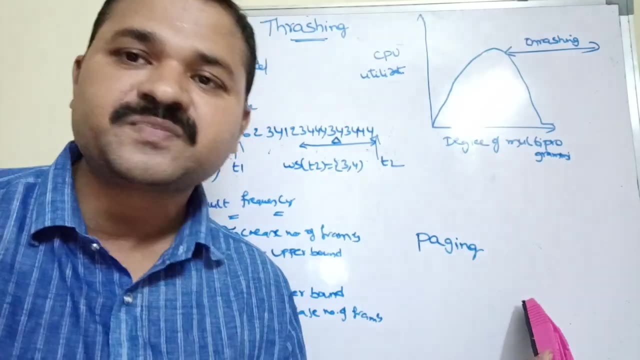 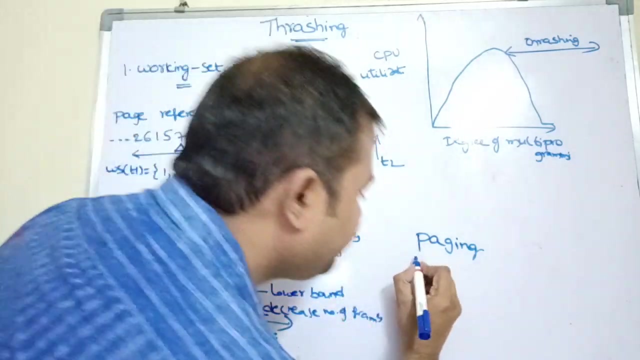 paging means swapping the pages between main memory and the secondary memory. So the definition for trashing is: if a process spends more time on paging rather than executing, then it is known as trashing. So let's see when the trashing will occur. Let me have a process: process people. 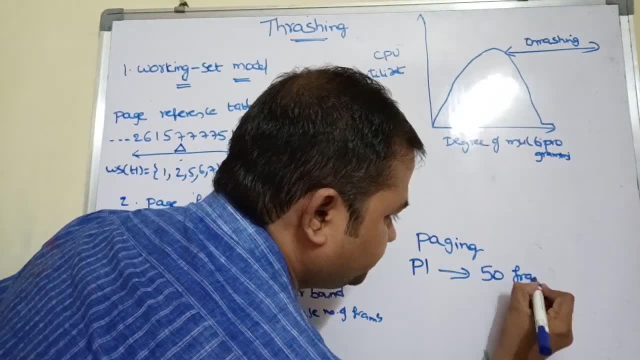 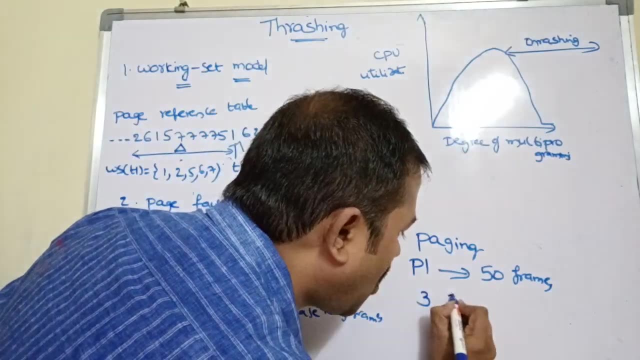 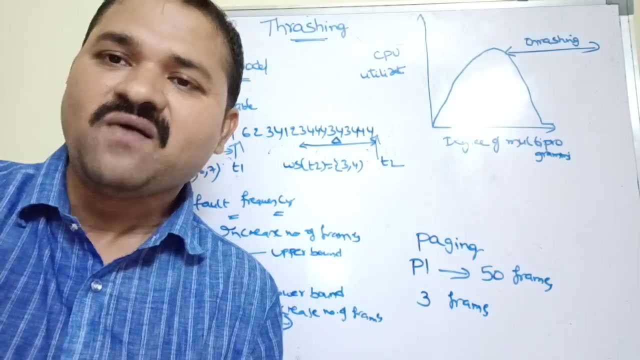 Let, process P1 requires 50 frames. So totally 50 frames are required for executing process P1. Whereas let us assume that operating system allocated only 3 frames to process P1. So that means here process P1 doesn't have enough number of frames for its execution. So what will happen? 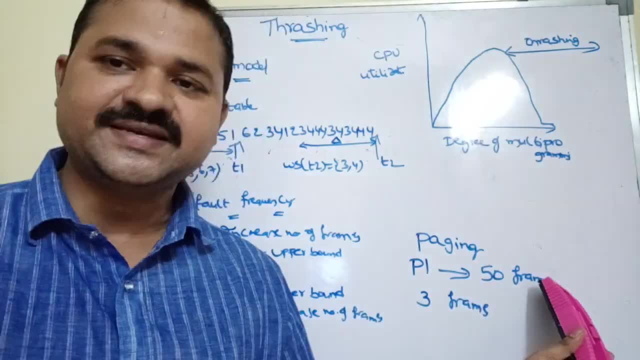 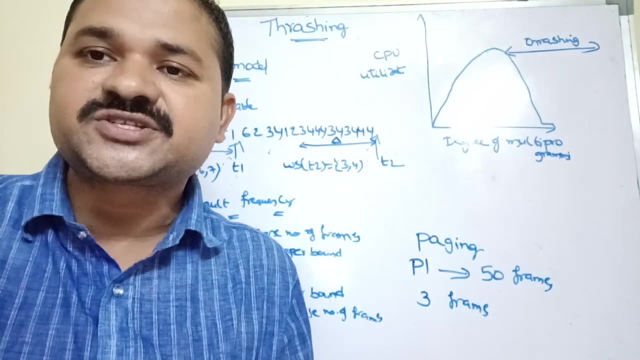 Too many page faults will occur. Why? Because here we have 50 pages whereas only 3 frames are allocated, So too many page faults will occur. So let's assume that operating system allocates only 3 frames to process P1. So if too many page faults occurs, then what will happen? We have to transfer, we have to swap the corresponding pages between the main memory and the secondary memory, So the CPU utilization will become less. Why? Because here the process is spending more time on paging, swapping rather than executing, So CPU utilization will become less. So what? 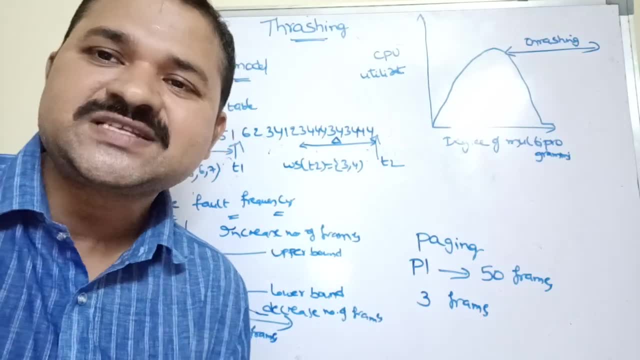 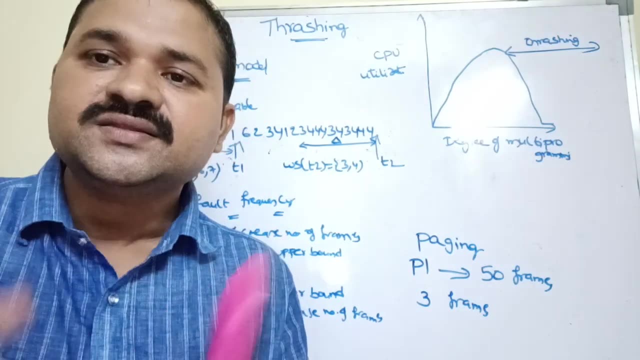 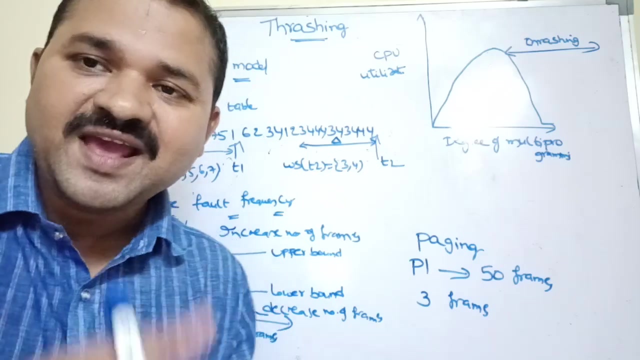 the operating system will think is main memory contains only limited number of processes, So that's why CPU utilization is low. So, in order to utilize the CPU in an effective manner, operating system replaces more number of processes in the main memory. So what will happen now? So, 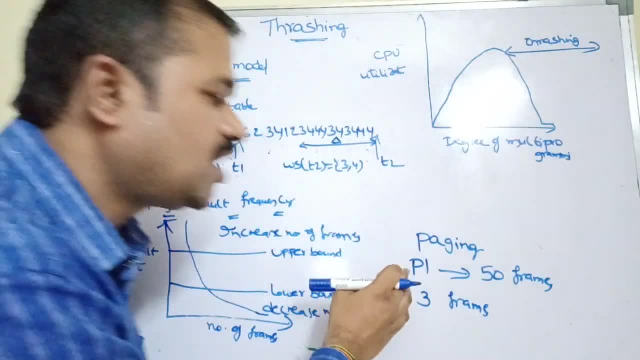 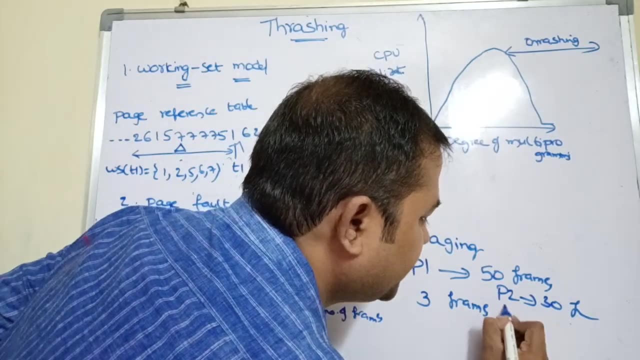 let us assume that two more processes are placed in the main memory. Let the demand for those processes is: let: process P2 requires 30 frames, whereas process P3 requires some 20 frames. So what is the demand of P1, P2, P3?? So 50 plus 30 plus. 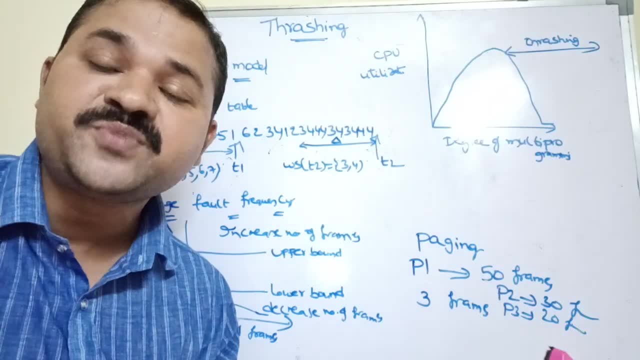 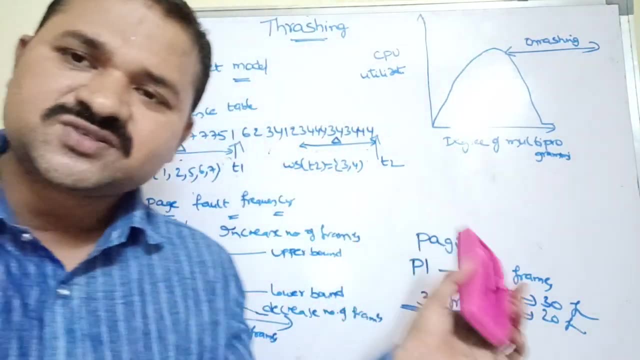 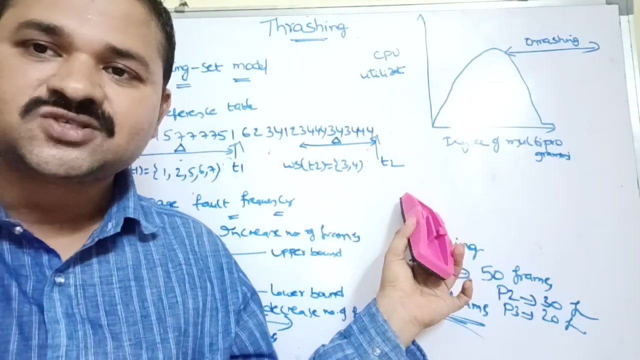 So 100 frames are needed for executing process P1, process P2 and process P3. Whereas operating system allocated how many frames? Only 3 frames. So what will happen? The page faults will become more and more and more So. this situation is known as trashing. So here what is the 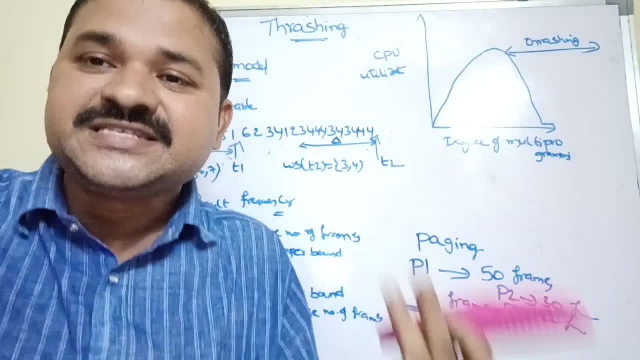 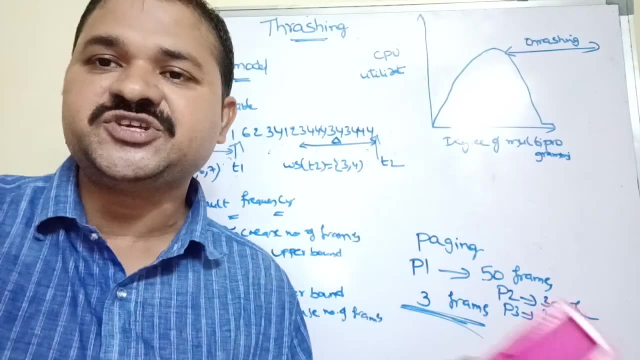 problem here. The process is spending more time on paging rather than executing, So this is known as trashing. So we can avoid the trashing, We can handle the trashing. So we can handle the trashing using two techniques. First one is working set model. Second one is: 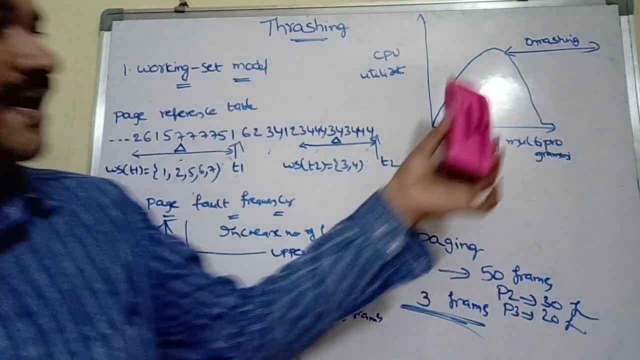 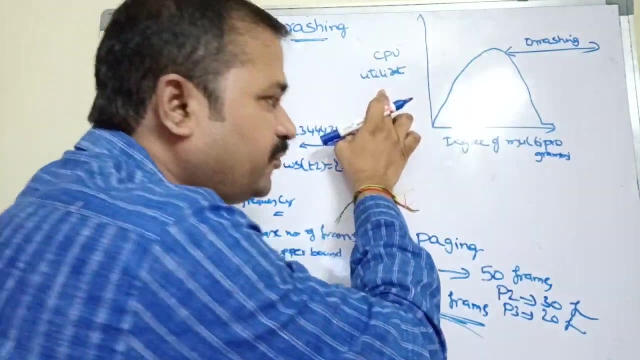 page fault frequency. So before discussing these techniques, let us see the diagram for trashing Here: x-axis represents degree of multiprogramming, Y-axis represents CPU utilization. So we know what is degree of multiprogramming. So degree of multiprogramming means placing more number of 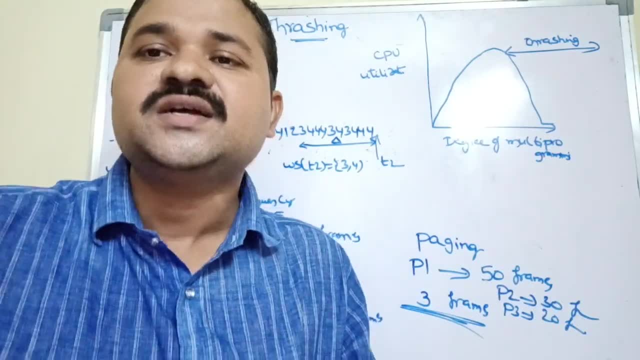 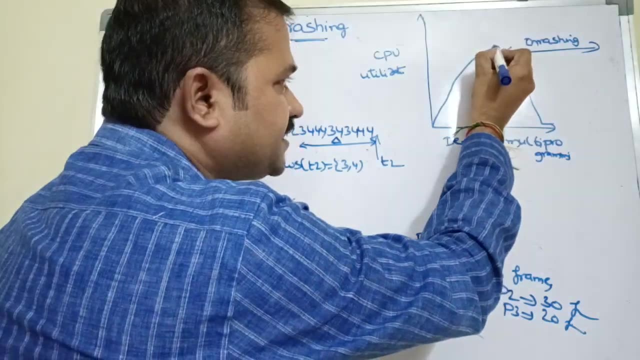 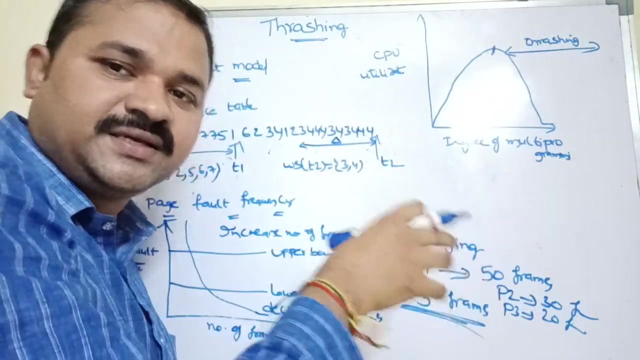 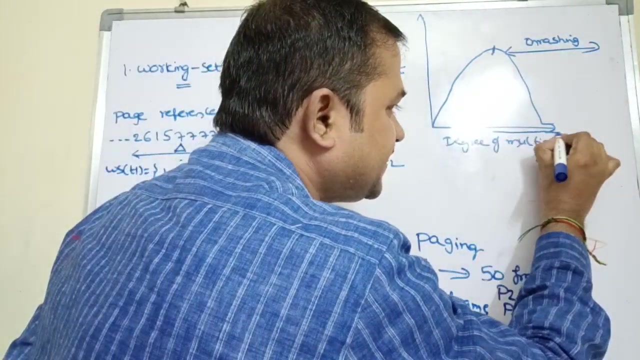 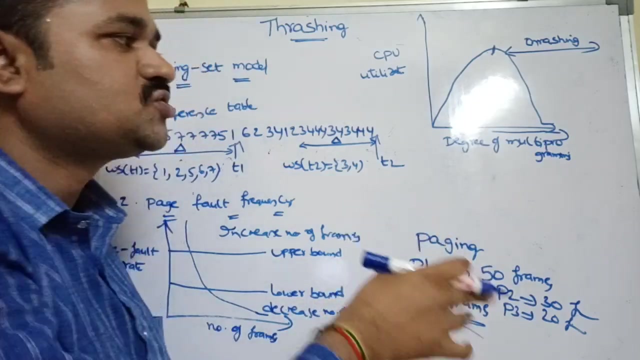 processes in the main memory in order to utilize CPU performance in an effective manner. So this is y-axis represents. So this is the example. we have just ninja put together. So five Storage devices are these things? One of my favorite development technology, Helica CPU Utilization. So up to this point. CPU utilization is excellent. But after that, let us assume that operating system places more number of processes in the main memory. So this is nothing but x-axis. After that, what has happened? let us assume that operating system places more number of processes in. 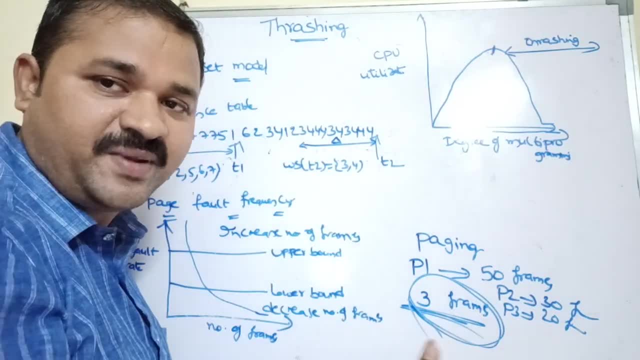 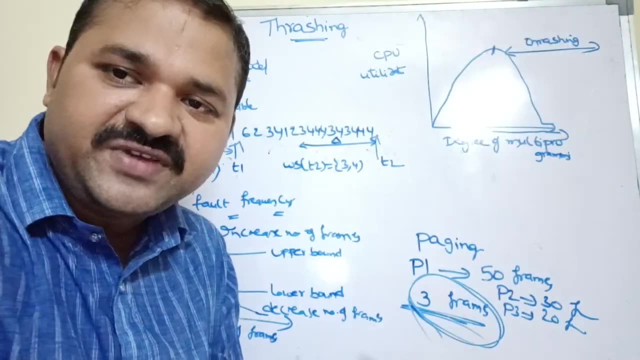 the main memory. So for those processes only less number of processes, less number of processes- frames were allocated. so what will happen now? base falls will become more so whenever base falls become more, then swapping will be needed between the primary memory and the secondary memory. so what we have in CPU realization: 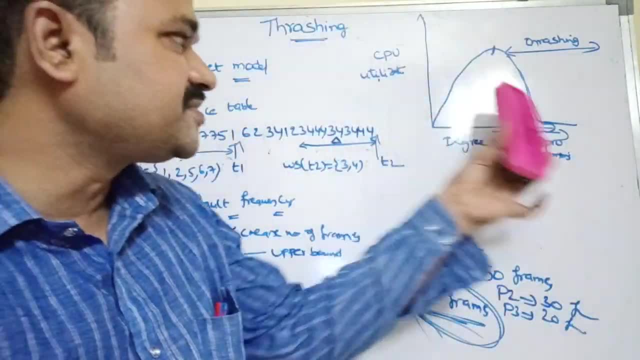 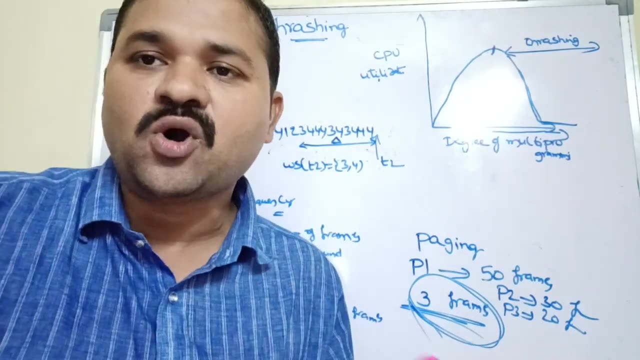 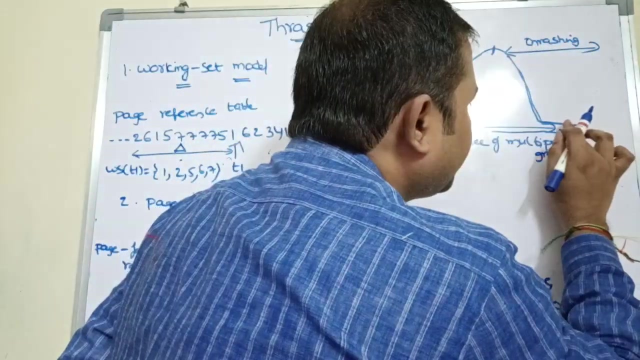 becomes drastically down. why it comes drastically down? why? because here the process is not spending time on executing, it is spending more time on the swapping the pages between primary memory and the secondary memory. so this, this portion, so this portion is known as trashing. so up to this point, the CPU